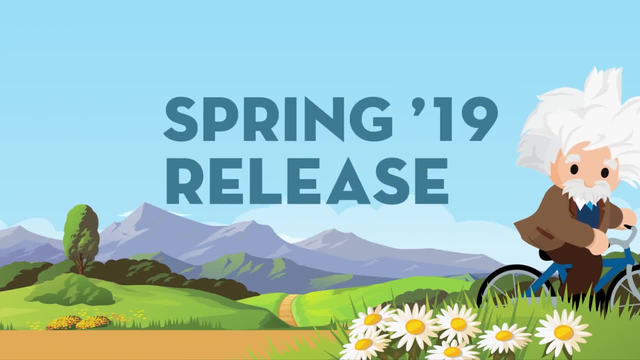 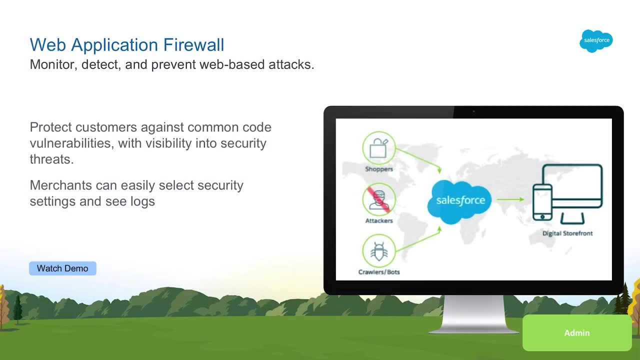 A web application firewall, or WAF, is an additional security tool for brands to protect against web security threats and common code vulnerabilities like SQL injection attacks, cross-site scripting and cross-site forgery requests. WAF is a new capability of the Commerce Cloud ECDN and shows our commitment to deepening the trust in our platform. 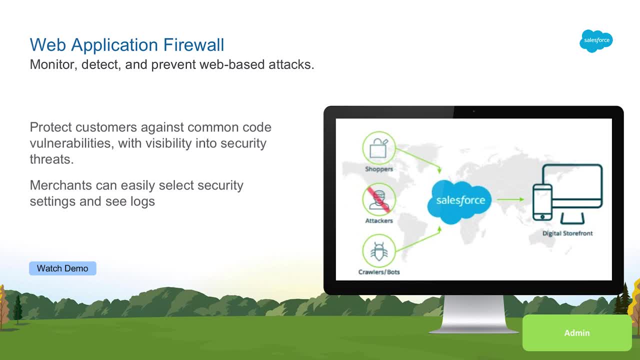 providing customers additional value at no extra cost, visibility into potential security threats and self-service ease of use. WAF examines all engagements within a merchant's site. These may be normal shopper actions, bot traffic or malicious requests. WAF performs a deep inspection of each request and filters out malicious traffic from real shoppers. 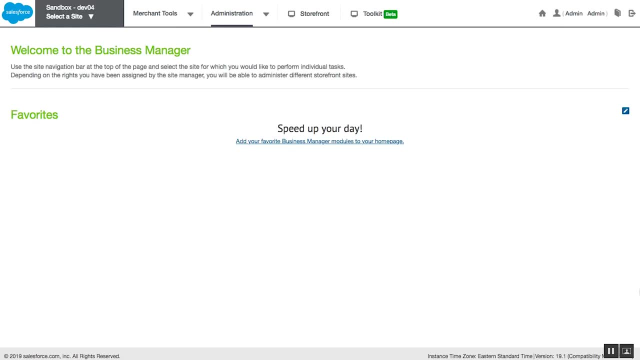 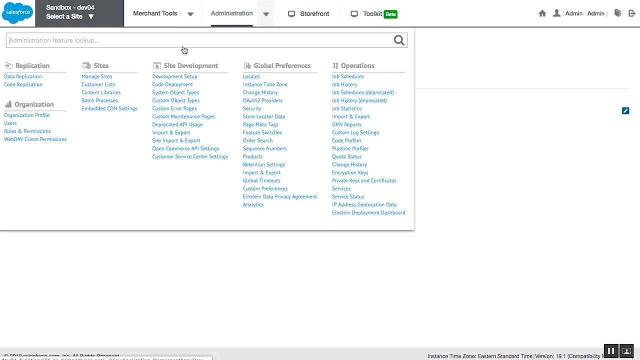 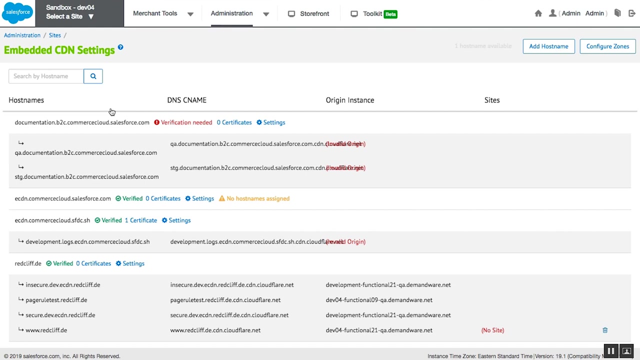 Merchants can access WAF directly from Business Manager. Let's show how. Navigate to Business Manager, Then select Administration Sites Embedded CDN Settings. In this case, our site is redcliffede. Click on the Settings button next to the redcliffede. 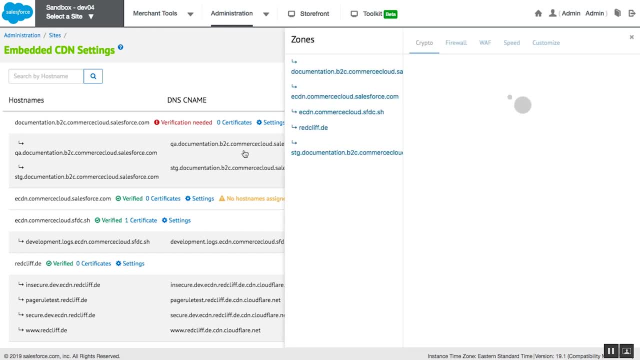 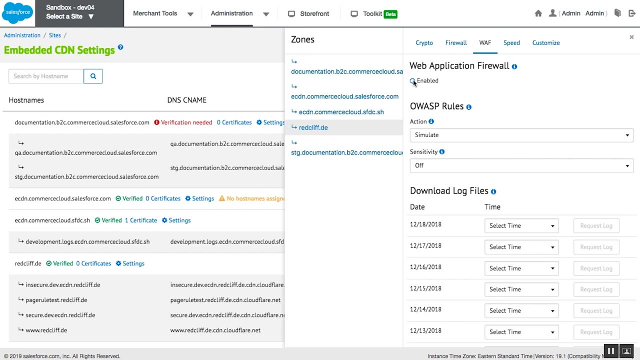 hostname. Here we can see a number of ECDN settings. Let's click on WAF. As this is our first time enabling WAF, we want to click the Enable button. Once WAF is enabled, we can see there are configurable rules based on the Open Web Application Security Project Standards. 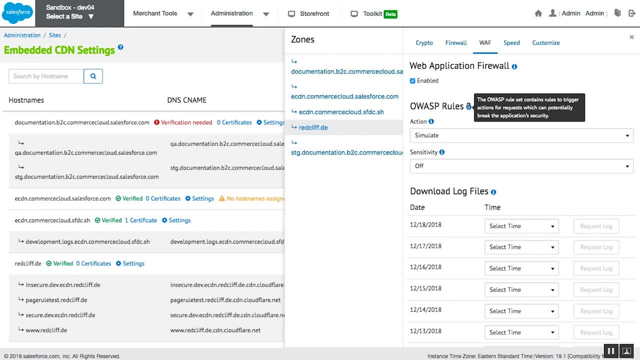 an international nonprofit organization dedicated to web application security. Merchants can select from three action modes in response to a threat detected. The following actions are Simulate: to simply log the event Challenge. to display a CAPTCHA challenge before the visitor can proceed. or Block Additionally. 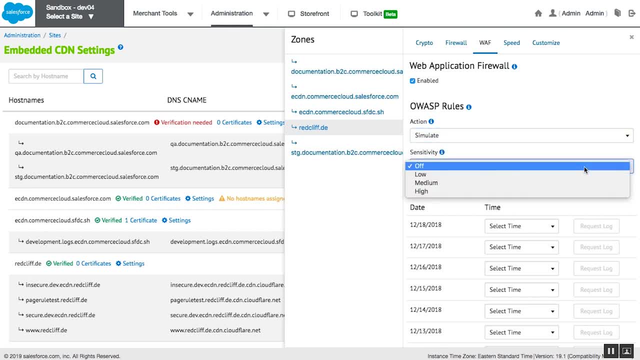 underneath we can see that WAF provides three sensitivity settings: High, Medium and Low. Lastly, merchants also have access to WAF logs, available in one-hour segments. The WAF logs contain reports of all ECDN traffic and enable customers to track things like IP address.